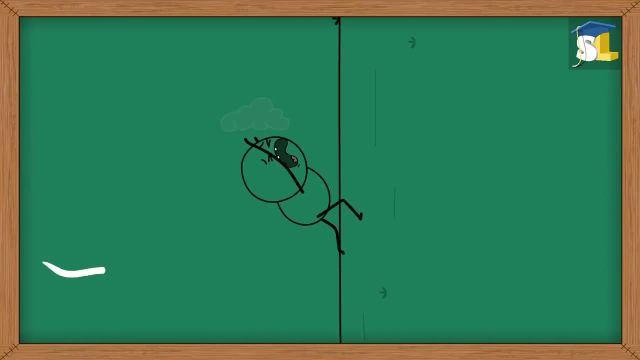 then the forces are said to be unbalanced. When a number of forces acting on an object are such that their resultant force is not equal to zero, then the forces are said to be unbalanced When a number of forces acting on an object are such that their resultant force is not equal to zero. 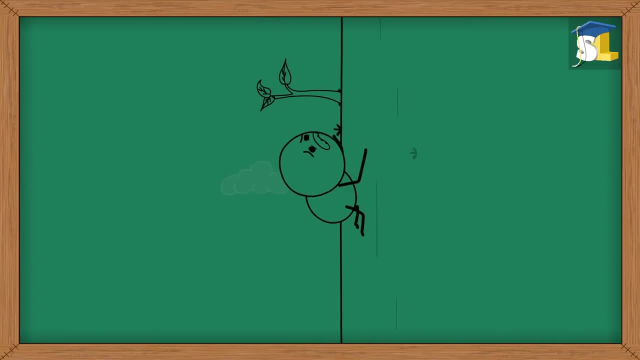 then the forces are said to be unbalanced. When a number of forces acting on an object are such that their resultant force is not equal to zero, then the forces are said to be unbalanced When a number of forces acting on an object are such that their resultant force is not equal to zero. 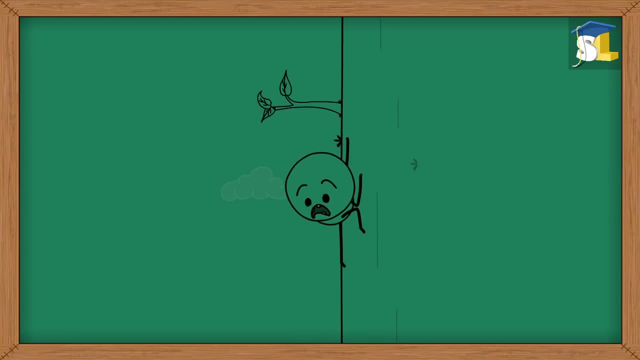 then the forces are said to be unbalanced. When a number of forces acting on an object are such that their resultant force is not equal to zero, then the forces are said to be unbalanced When a number of forces acting on an object are such that their resultant force is not equal to zero. 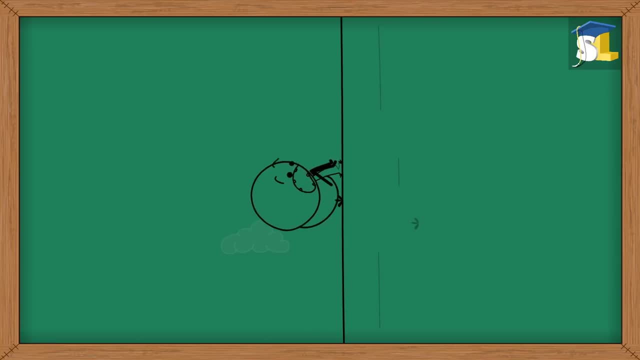 then the forces are said to be unbalanced. When a number of forces acting on an object are such that their resultant force is not equal to zero, then the forces are said to be unbalanced When a number of forces acting on an object are such that their resultant force is not equal to zero. 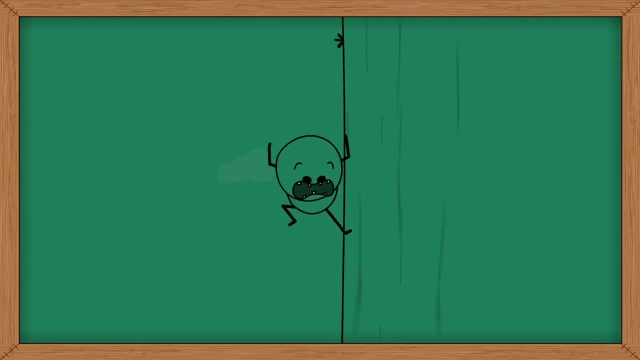 then the forces are said to be unbalanced. When a number of forces acting on an object are such that their resultant force is not equal to zero, then the forces are said to be unbalanced When a number of forces acting on an object are such that their resultant force is not equal to zero. 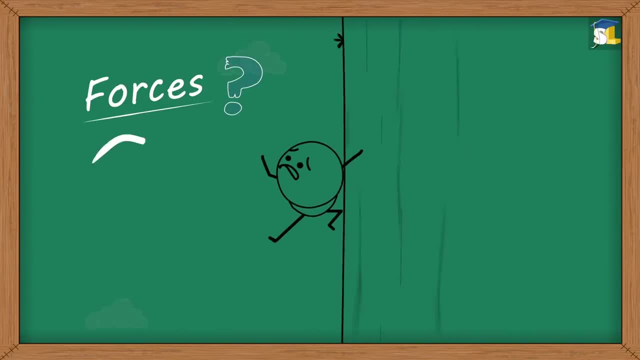 then the forces are said to be unbalanced. When a number of forces acting on an object are such that their resultant force is not equal to zero, then the forces are said to be unbalanced When a number of forces acting on an object are such that their resultant force is not equal to zero. 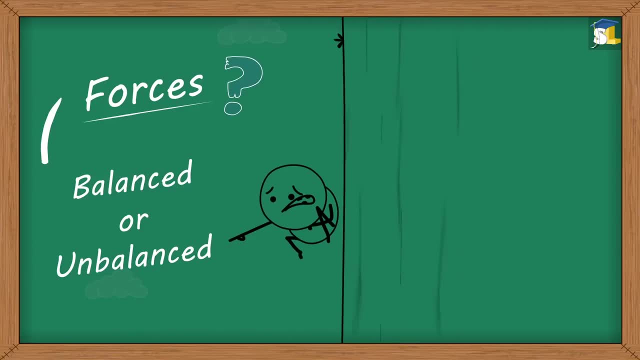 then the forces are said to be unbalanced. When a number of forces acting on an object are such that their resultant force is not equal to zero, then the forces are said to be unbalanced When a number of forces acting on an object are such that their resultant force is not equal to zero. 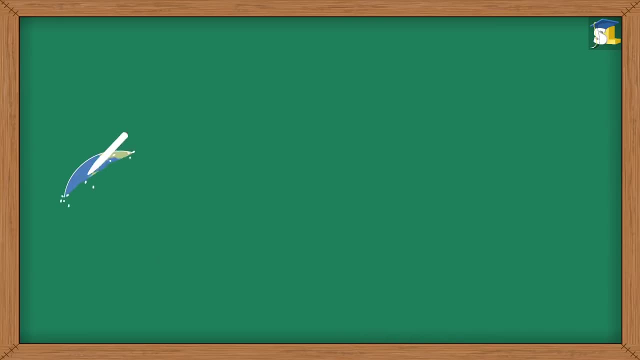 then the forces are said to be unbalanced. When a number of forces acting on an object are such that their resultant force is not equal to zero, then the forces are said to be unbalanced When a number of forces acting on an object are such that their resultant force is not equal to zero. 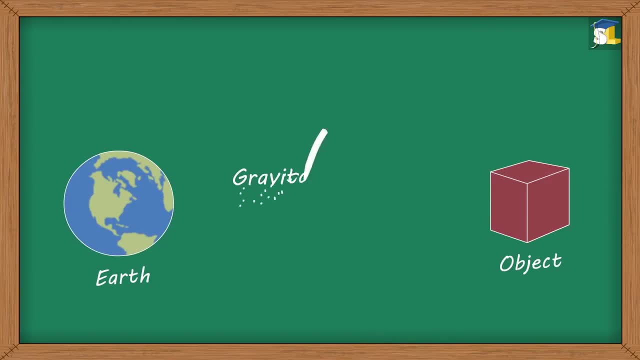 then the forces are said to be unbalanced. When a number of forces acting on an object are such that their resultant force is not equal to zero, then the forces are said to be unbalanced When a number of forces acting on an object are such that their resultant force is not equal to zero. 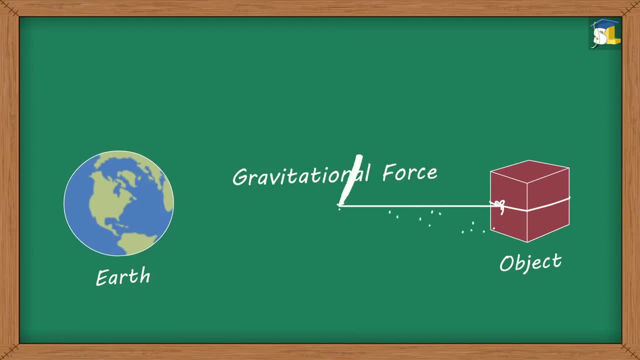 then the forces are said to be unbalanced. When a number of forces acting on an object are such that their resultant force is not equal to zero, then the forces are said to be unbalanced When a number of forces acting on an object are such that their resultant force is not equal to zero. 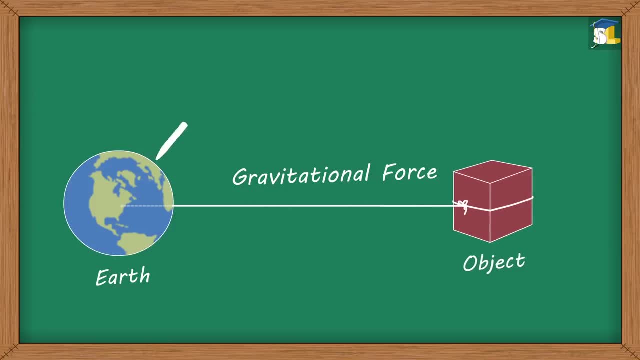 then the forces are said to be unbalanced. When a number of forces acting on an object are such that their resultant force is not equal to zero, then the forces are said to be unbalanced When a number of forces acting on an object are such that their resultant force is not equal to zero. 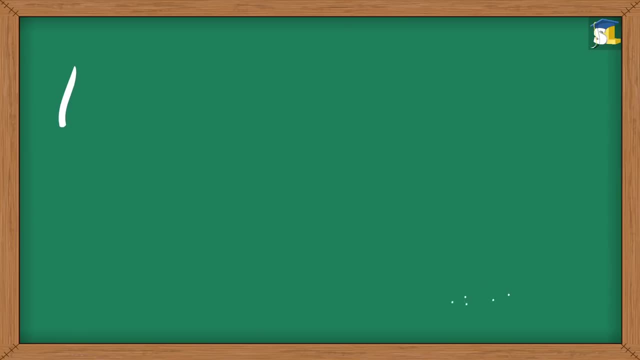 then the forces are said to be unbalanced. When a number of forces acting on an object are such that their resultant force is not equal to zero, then the forces are said to be unbalanced When a number of forces acting on an object are such that their resultant force is not equal to zero. 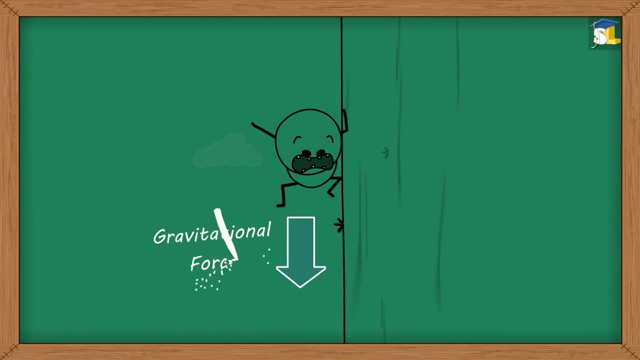 then the forces are said to be unbalanced. When a number of forces acting on an object are such that their resultant force is not equal to zero, then the forces are said to be unbalanced When a number of forces acting on an object are such that their resultant force is not equal to zero. 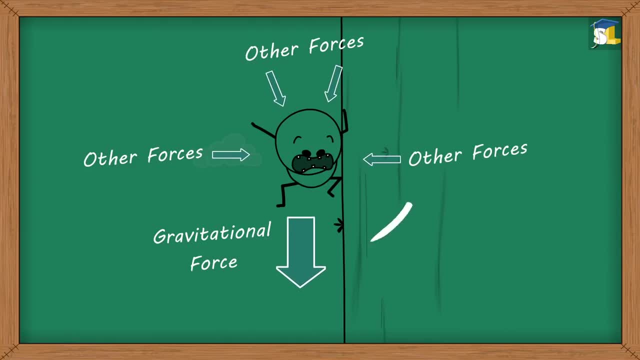 then the forces are said to be unbalanced. When a number of forces acting on an object are such that their resultant force is not equal to zero, then the forces are said to be unbalanced When a number of forces acting on an object are such that their resultant force is not equal to zero. 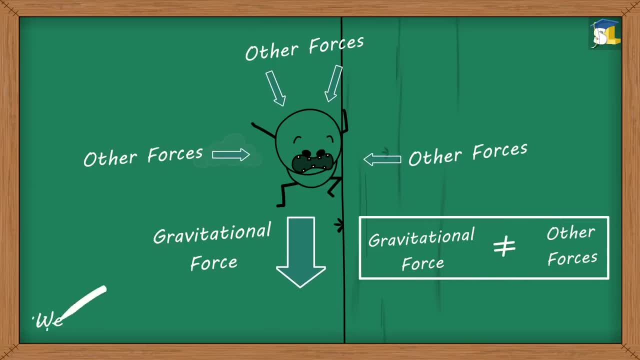 then the forces are said to be unbalanced. When a number of forces acting on an object are such that their resultant force is not equal to zero, then the forces are said to be unbalanced. So from this sense, we can conclude. So, from this sense, we can conclude.